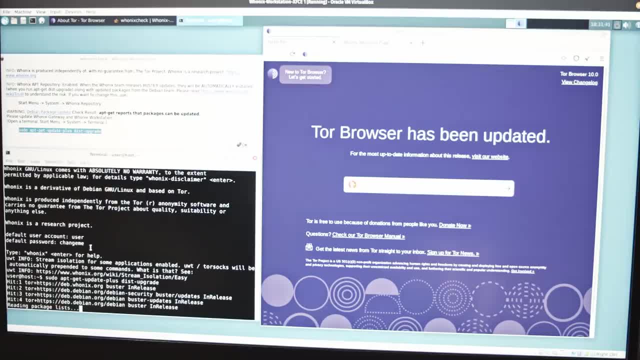 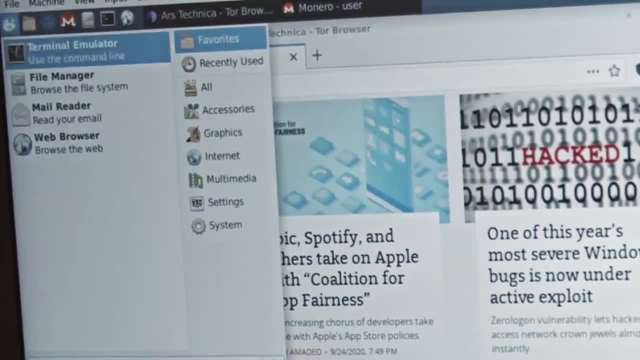 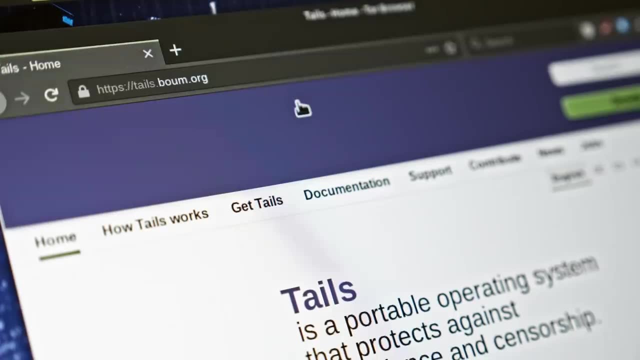 Even with full device encryption, memory locks can often easily be recovered by an adversary with physical access to your device. Not everyone has the luxury of physical security, and some people just have to assume that their computer will likely fall into the wrong hands. This is why security experts with strong sense for protecting human rights in the digital world 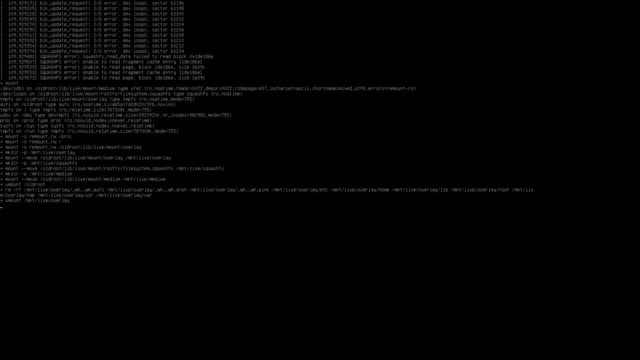 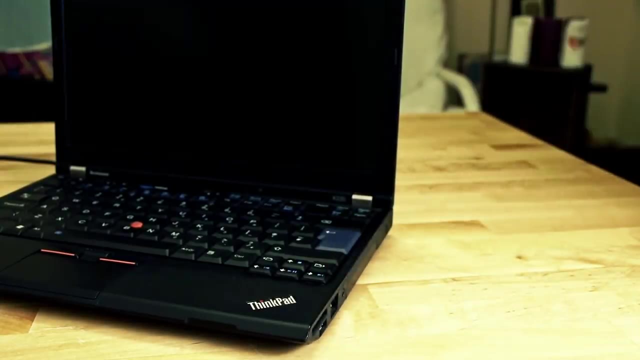 have been working on creating a system that doesn't remember anything about itself, A system that forensically wipes all evidence of its use immediately after a user ends their session, A system that looks exactly the same no matter who uses it or for what purpose. 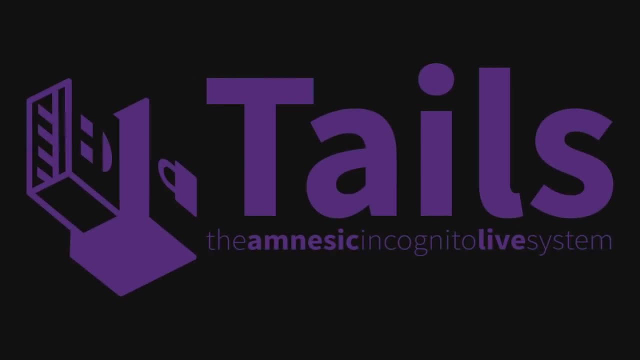 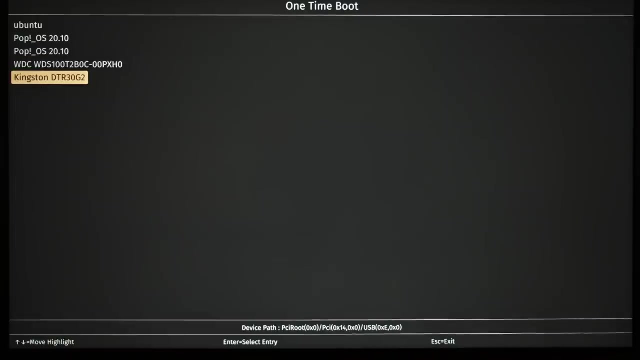 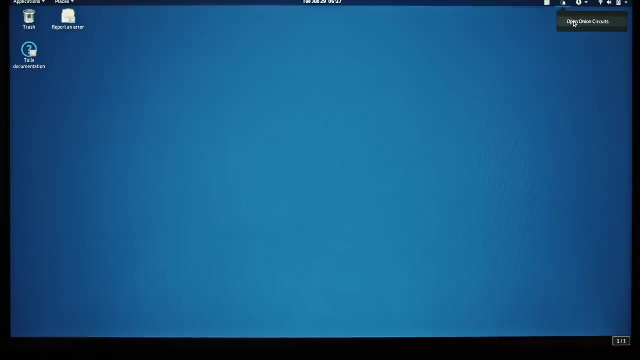 And now such a system has a name: Tails The Amnesic Incognito Live System. Live system because it's an operating system designed to run off of a USB flash drive instead of being permanently installed on an internal drive. Incognito because its entire traffic is routed through Tor. 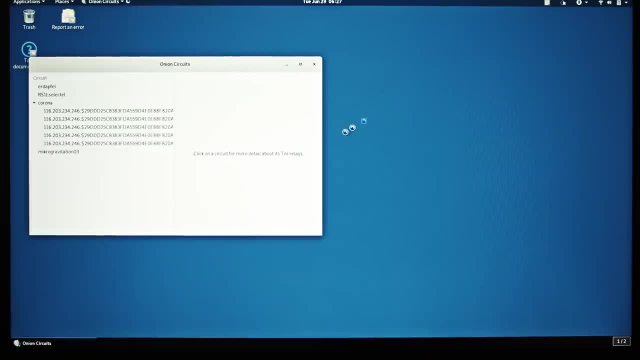 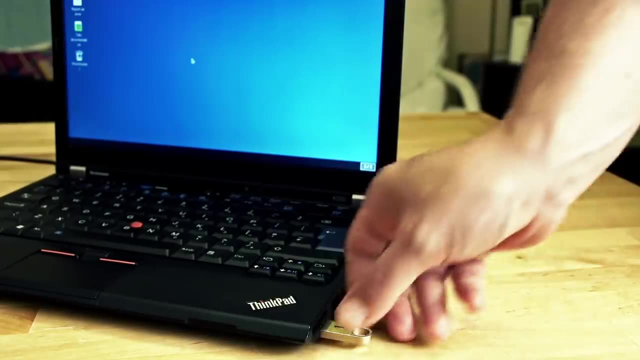 and the default fingerprint of each Tails installation matches perfectly with every other Tails user on the planet. Amnesic means: every time you reboot, plug out your USB or shut down, all the information about your session activities is wiped from the USB. 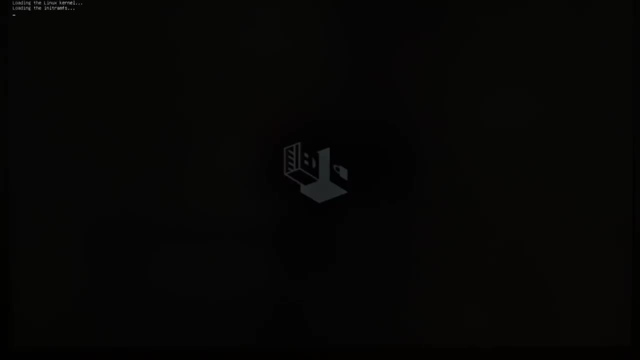 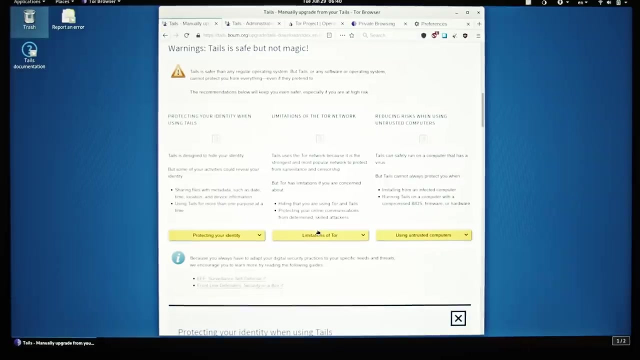 The Amnesic Incognito Live System is designed to be able to run on a USB flash drive as well as from the host memory. This forensic erasure leaves no files on the host system whatsoever. Tails is a security application and as such, it's not just about the tool itself. 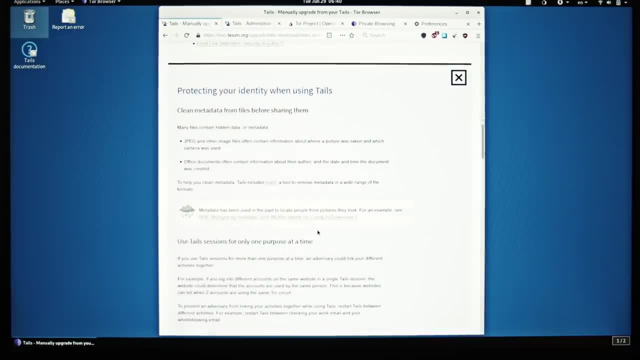 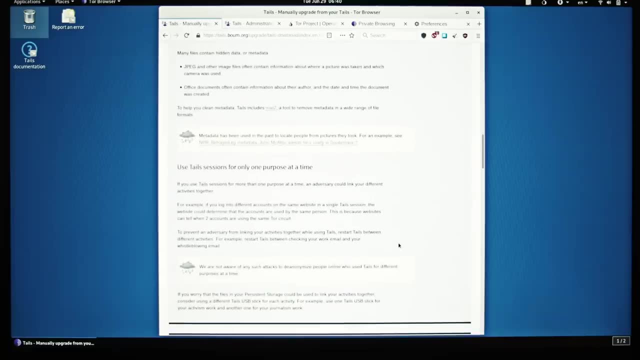 but also about your operation security. How you obtain, use and maintain Tails for your particular situation can make or break your security. No security tool can do everything for you. If you want to make the most out of Tails, you have to educate yourself about the security. 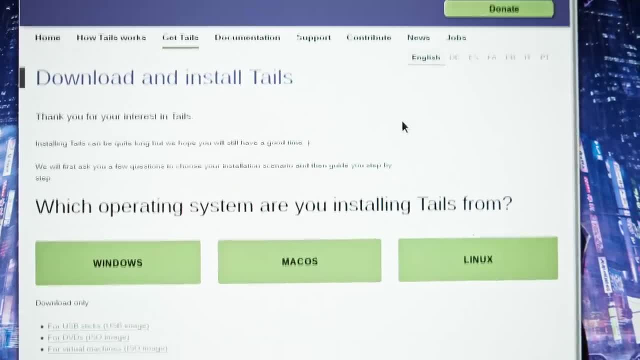 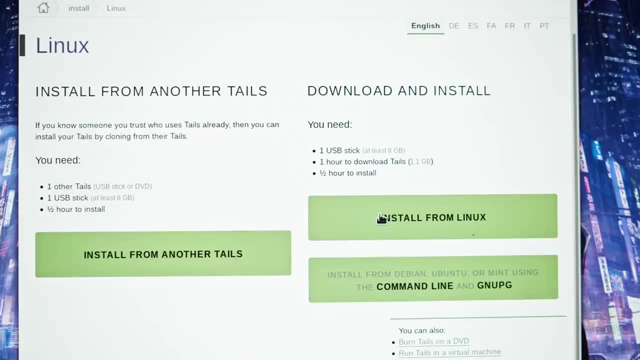 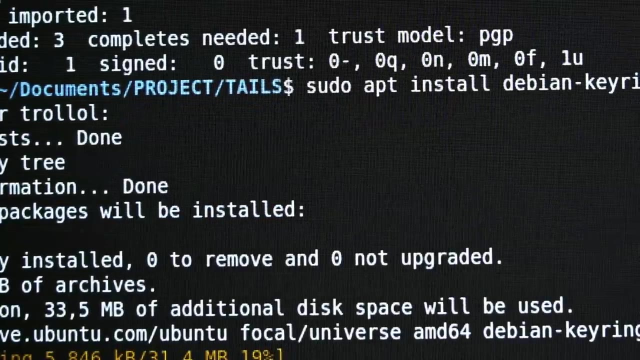 of using Tails and Tor in general. This tutorial will guide you through the official Tails installation process, as maintained at the time of making of this video. Use this tutorial as a reference only and always follow the official guidelines for maximum security. The aim of this tutorial is to provide novice users with visual experience of installing. 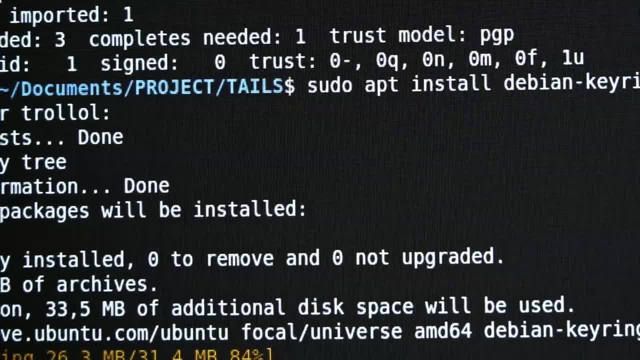 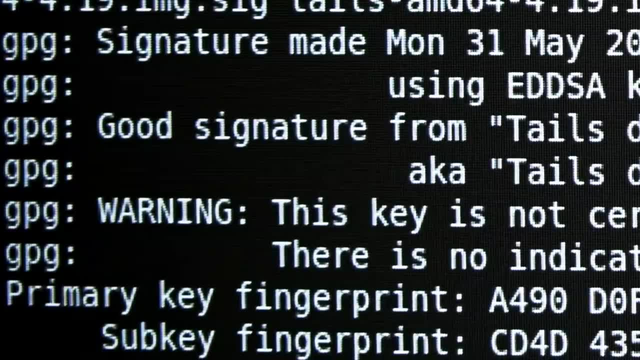 and using Tails in order for you to know what to expect when going through the process yourself. If your life depends on strong anonymity and security, you need to acquire education and skills beyond the scope of this video. Consult with a certified or accredited security professional if you need to. 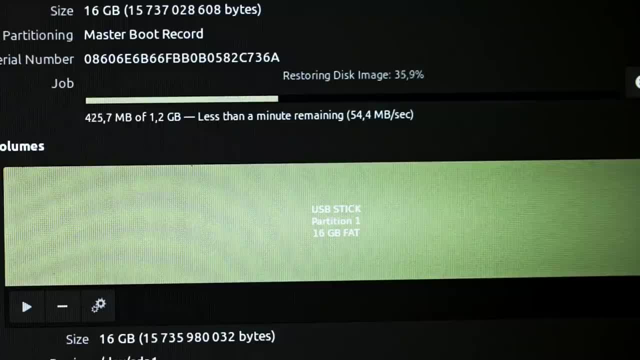 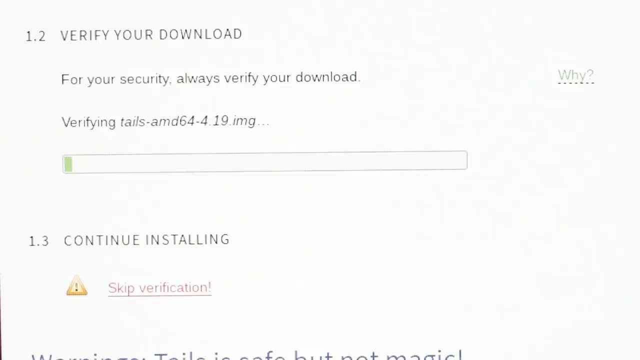 Now let's go over what this Tails tutorial will cover. I'll show you how to obtain Tails image alongside different methods of security verification. Choose your own method, but don't skip verification completely, Otherwise you have to blindly trust your Tails isn't compromised. 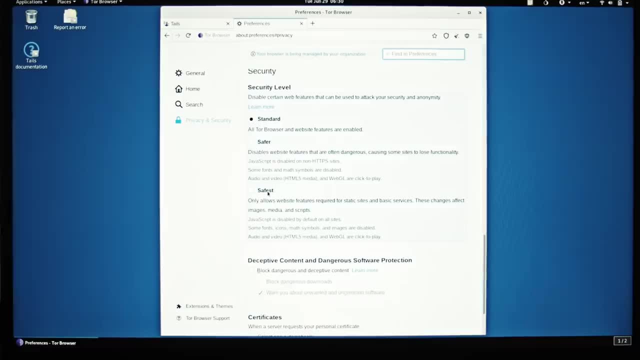 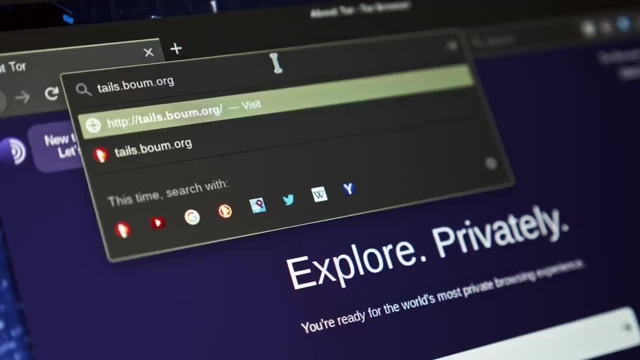 We'll go over a few important OPSEC points to consider before flashing the image on a USB drive and booting into Tails. So let's begin. The official website for Tails is wwwtalescom. The website for Tails is wwwtalesboumorg. 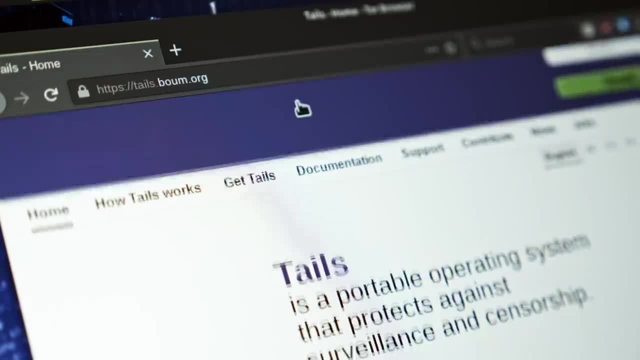 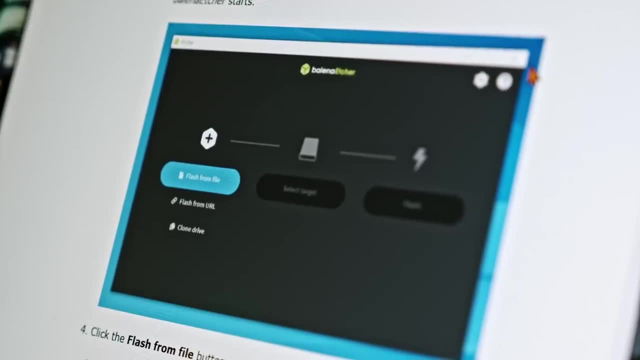 You can access it from Tor browser for additional anonymity when obtaining Tails. What I love about Tails as a project is that it is really approachable to novice users, and that's how it should be. Security shouldn't be just the privilege of experts. 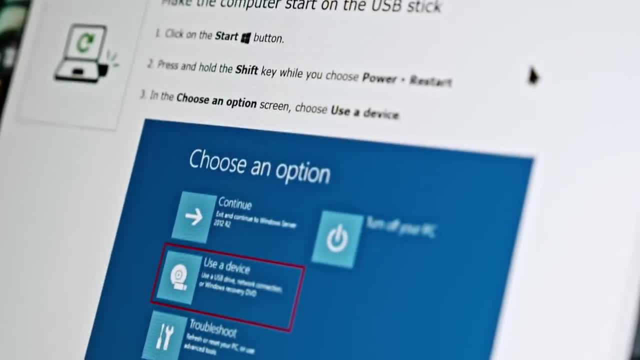 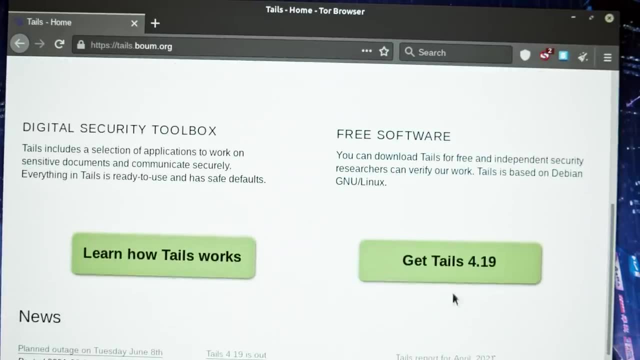 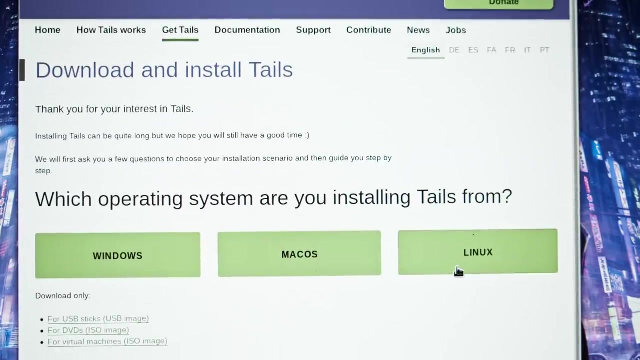 Journalists, activists and regular nontechnical people need anonymity and security too, and that's whom Tails is targeted towards. Click on Get Tails and choose which operating system you'll be installing from. on any system, but the installation instructions slightly vary depending on your host os. i'll 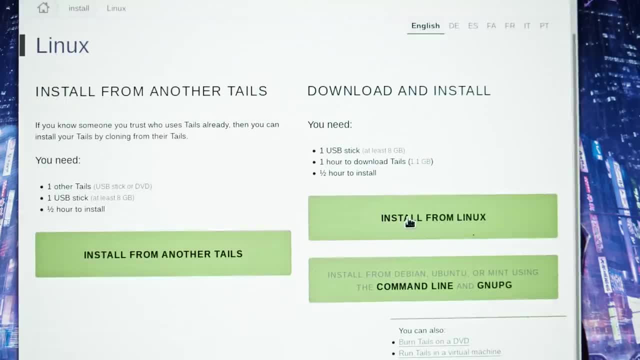 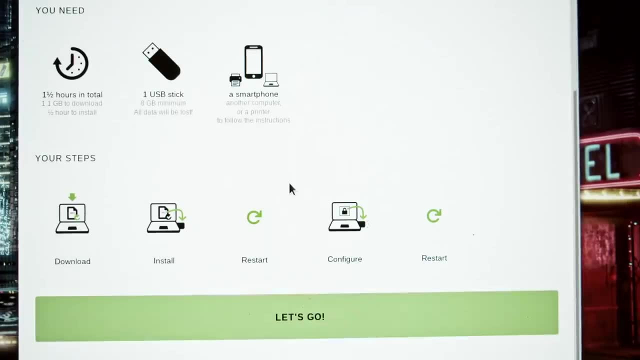 choose linux because that's what i'm using, but instructions for windows and mac os have only minor differences and i'll point them out throughout this video. make sure to read the instructions carefully to know what you need for your tails installation. grab a usb stick with at. 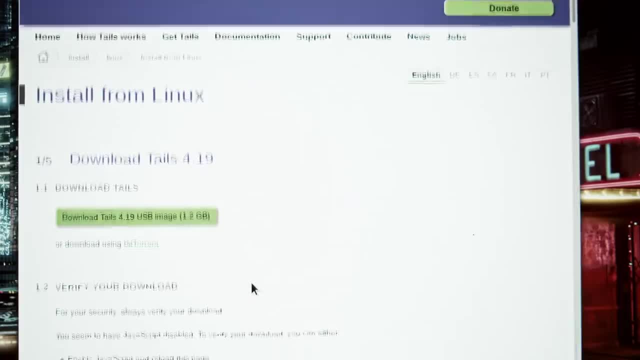 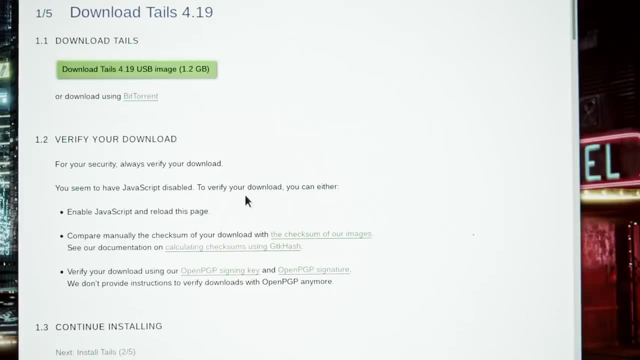 least 8 gigabyte capacity and continue to the next step. now you get to choose how you want to download tails, and this might determine the next verification steps. be aware you should never skip verification and choose at least one of the following methods, whether you download details. 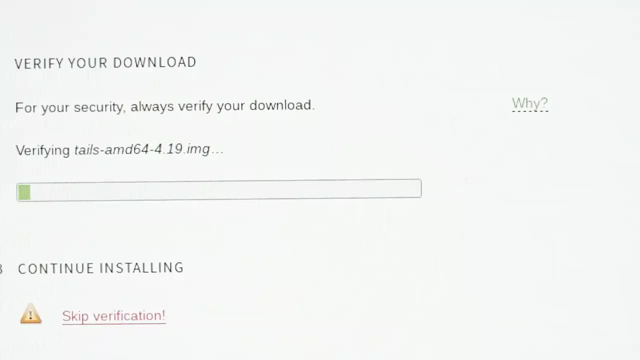 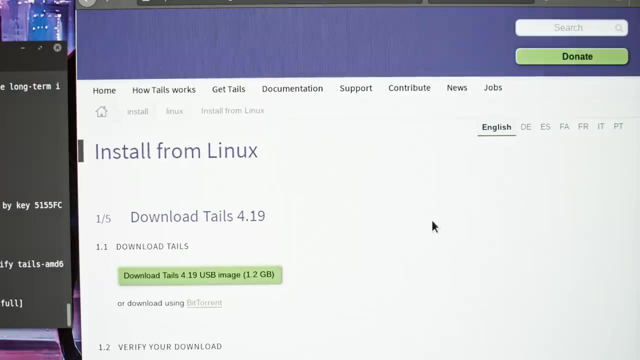 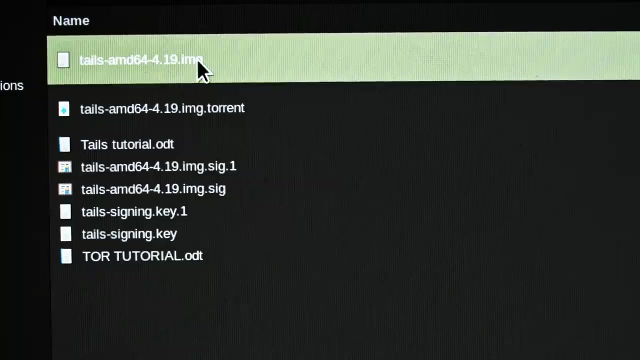 directly from a mirror link or through bit torrent. you should use tails verification utility. this requires that you enable javascript, but this method provides a simple, cross-platform and user-friendly technique to verify tails images. the only limitation of javascript verification is when facing advanced adversaries, an attacker would have to perform a manual middle attack. 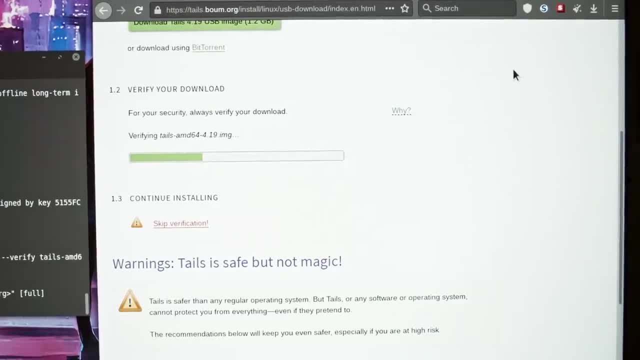 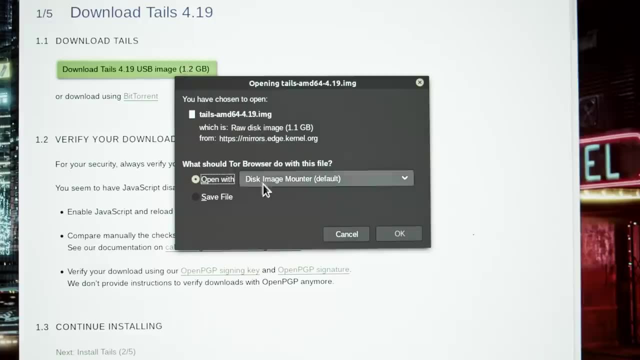 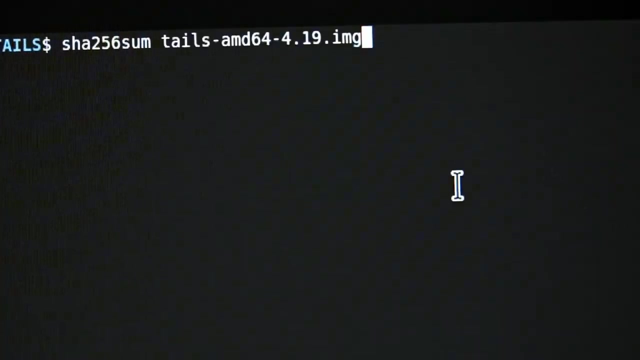 or compromise tails website or servers covertly without the tail project noticing. additionally to this, you can verify checksum of image files. if you download a tails image using a mirror link, you'll need to manually check for sha sums. linux has sh, a verification tool built into the command line, which makes it more secure than obtaining a. 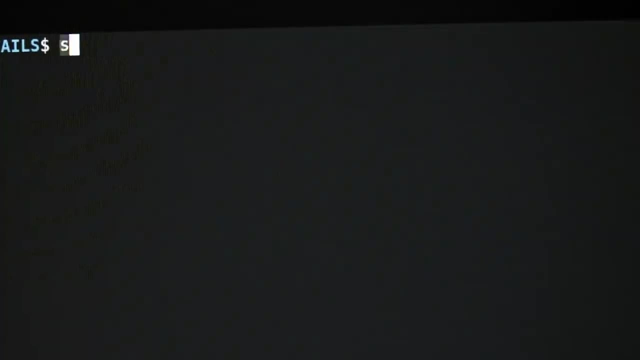 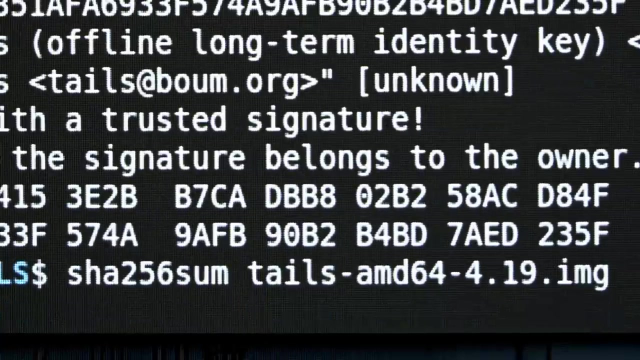 third-party checksum tool on windows and mac. the simple command is sha256 sum, followed by a single space and then full name of the downloaded tails image file. make sure your terminal is navigated in the directory of your tails files. the utility will generate a string that has to match. 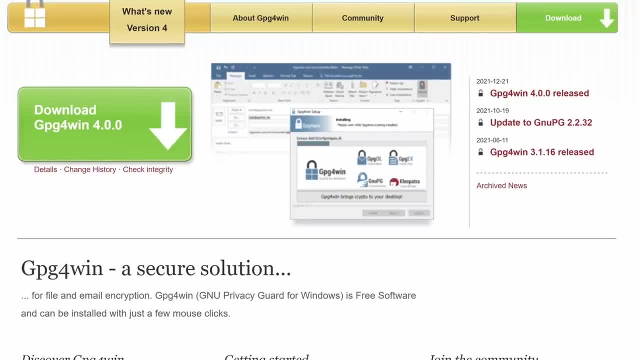 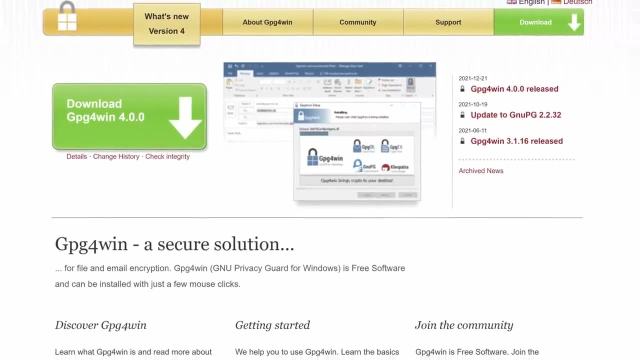 perfectly with the one available on the tails website. if you want to check some on windows, you can create a checksum file for the tails image using gpg for win utility and then comparing the output. an alternative method is to download tails torrent file. it already includes a checksum for. 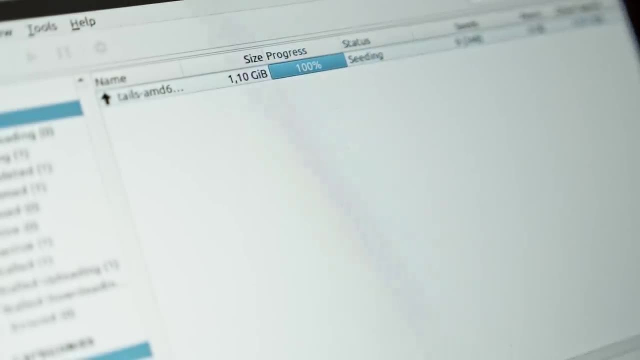 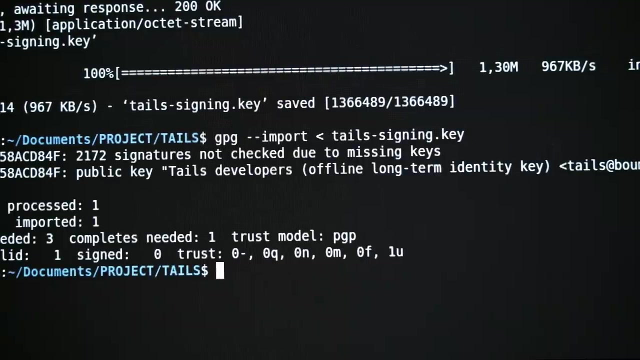 the image and your big turn client will automatically verify when the download finishes, so you can use the checksum file to verify the image and then compare the image file with the image file. so the next step is to manually verify openpgp signatures if you don't have an advanced 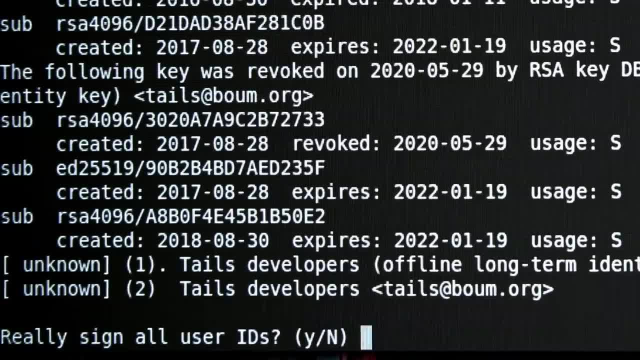 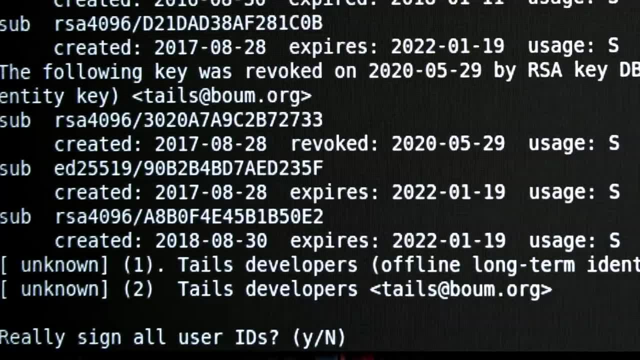 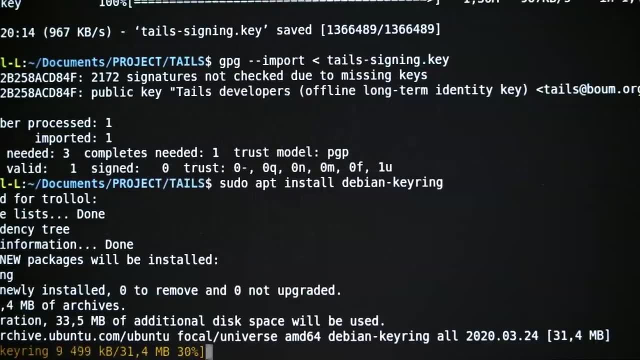 knowledge of openpgp. this method does not provide more security than the javascript verification utility, but if you're running a debian based linux distribution, you can follow the command line installation instructions for linux. since debian derivatives ship with trusted openpgp keys by default, you can proceed with openpgp steps by simply copying the commands from the instructions. 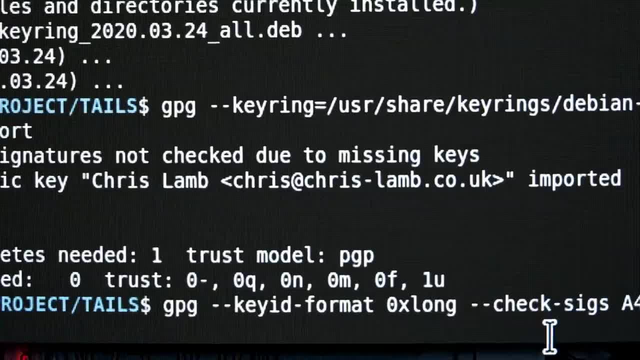 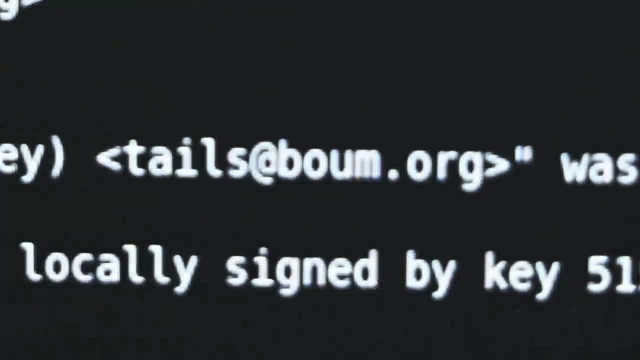 and debian developers. the fourth step checks for verification of the tail signing key, where you need to look for this specific line in the output. only then you can verify the tail signing key with your own key. if you've never used openpgp before, you may need to generate your own signing key. the 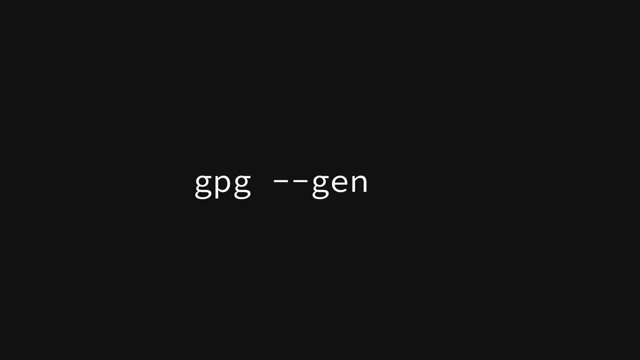 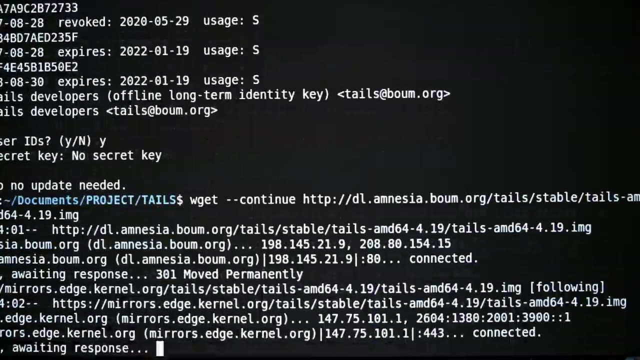 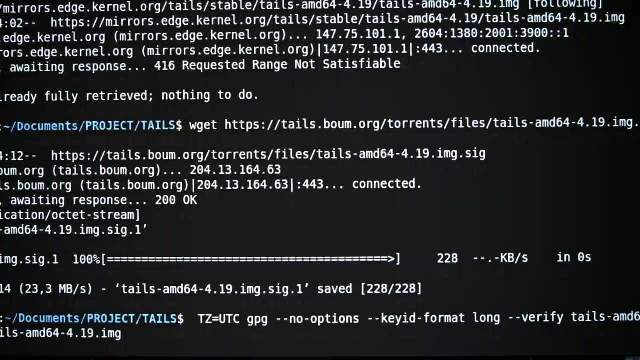 command for this is gpg, space, double dash, gen dash key and then follow the instructions on the screen. if you already download a tails image, you can skip the first command in the download section and get the tails image in the last step. verify. the tails image is signed by the tail signing key with the. 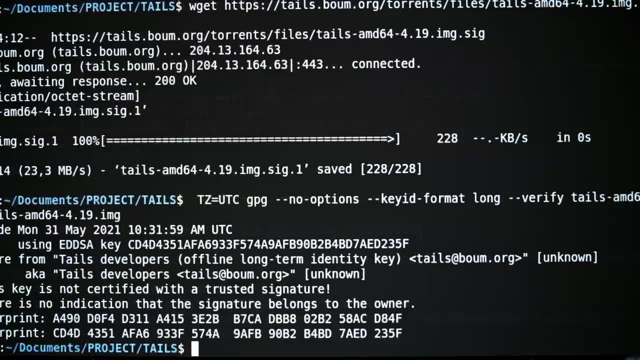 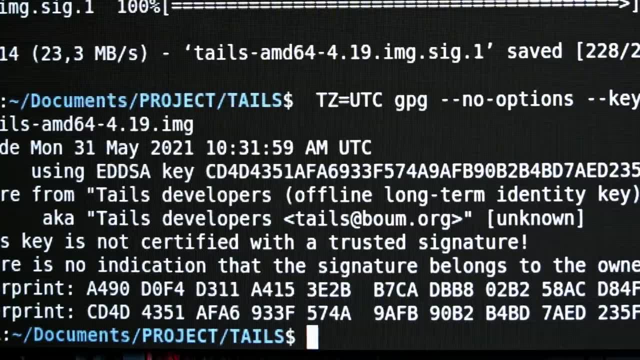 following command. the output you should get looks like this. it should contain the key id and align with a good signature from tails developer. it is possible to complete openpgp verification without generating your own key, but you will get a warning: it's not certified and there is no indication it. 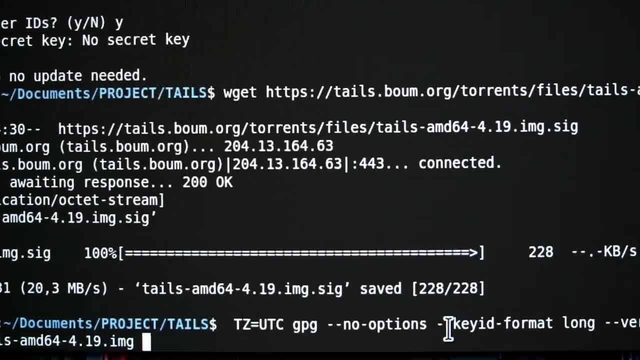 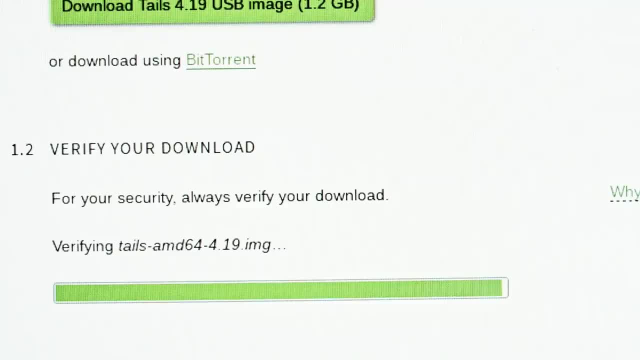 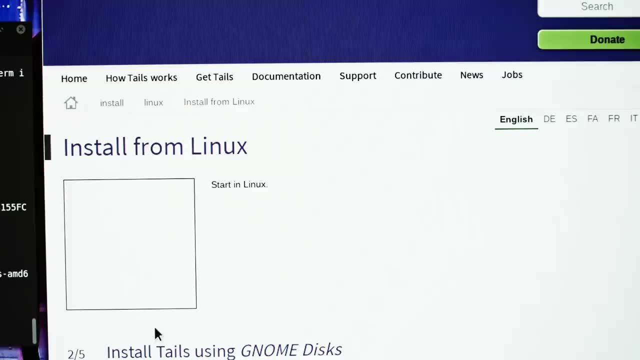 belongs to the owner. if the tails image is in any way compromised, the output of the verification will say bad signature and you shouldn't use this image to install tail signals. if the verification went through, you are ready to flash tails on your usb stick. this process is very simple on all platforms. on linux you can use the built-in gnome disk utility by. 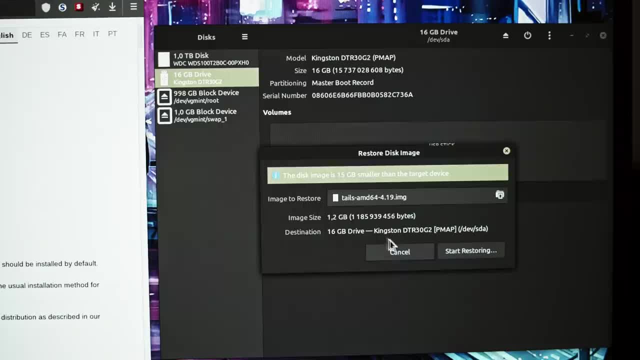 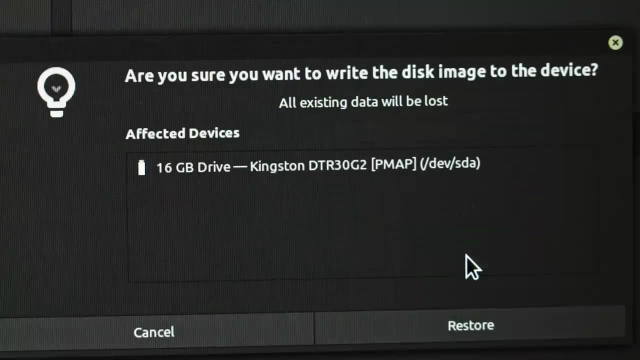 choosing restore disk image option for your usb drive, make sure you select the correct drive, because this will erase all of its data. make sure to maintain backups, because you won't be able to recover your data if you make a mistake. on windows and mac, you can use a simple etcher utility. where 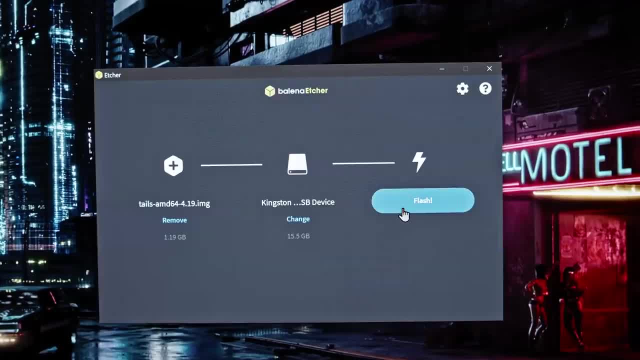 you can select the tails image, your usb drive will be able to recover your data if you make a mistake. on windows and mac, you can use the simple etcher utility, where you can select the tails image your usb drive and flash. it's simple, but the same precautions apply. make sure to backup your 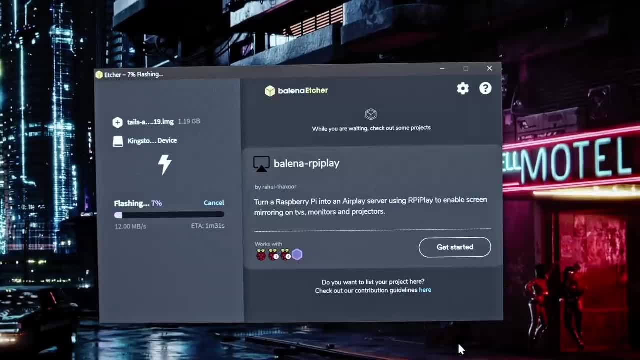 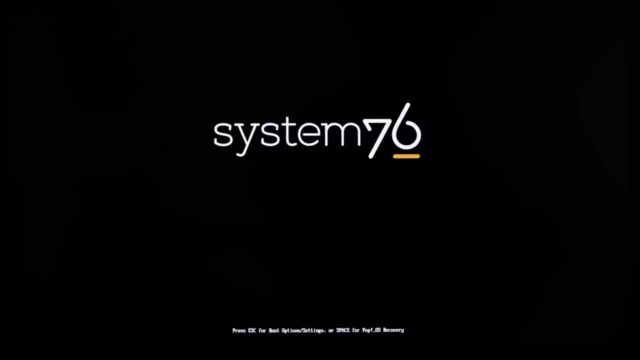 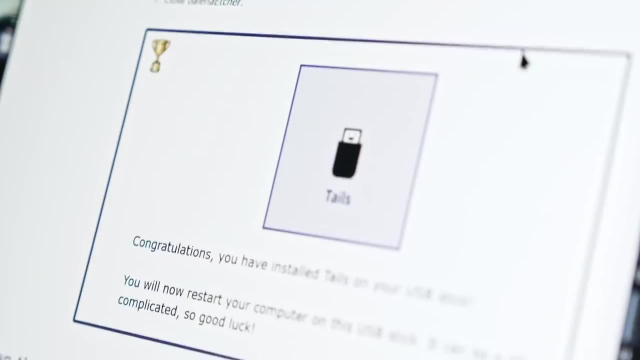 content, because this will erase all the data from your usb stick. after flashing the image, you're ready to boot to tails. for the first time to boot to tails, you need to know how to access your machine's boot menu or bios settings. this is usually a matter of pressing escape f2, f11 or f12. 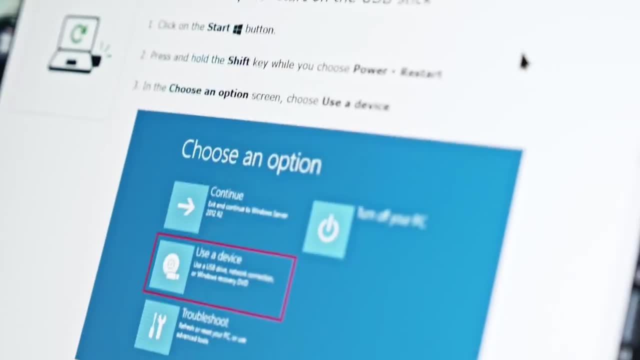 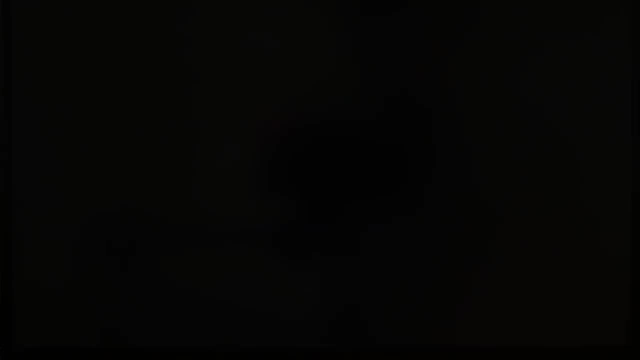 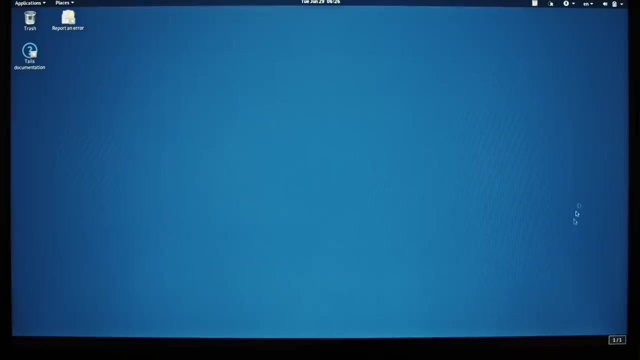 on windows 10. you can get to the bios through update and security settings. if you're not sure, follow the official instructions. once tails boots up, select your language, keyboard and formats, and start tails. it should take less than a minute for the desktop to appear. one of the first issues you may encounter is network. 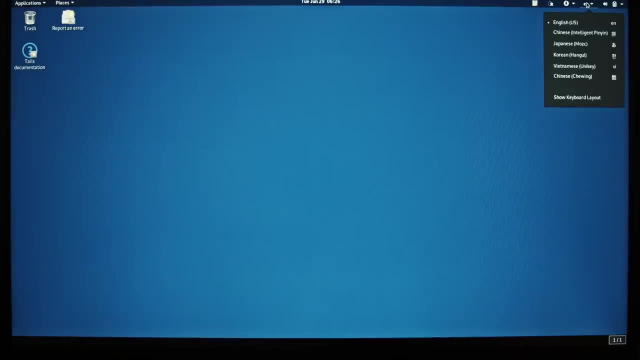 connectivity. linux in general is not the best friends with wi-fi cards, and tails is no exception. if your wi-fi interface is not available at all, use an ethernet cable or get a working usb wi-fi adapter for about 10 to 15 dollars. one additional step you can take, but this is 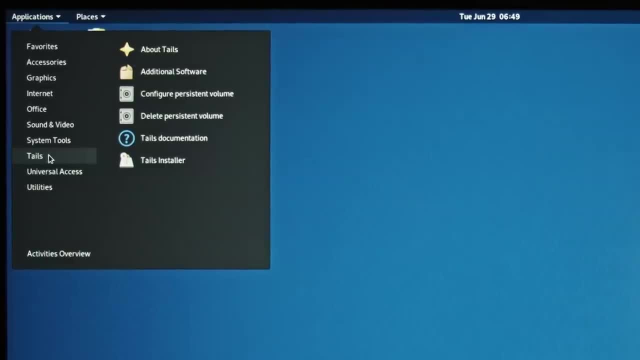 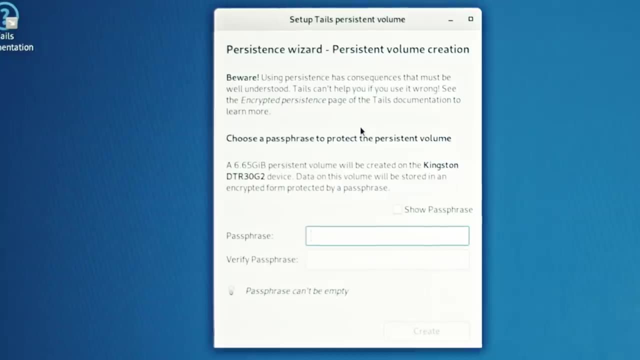 entirely optional is to create an encrypted persistent storage. this is only in case you need to securely store files on your usb drive. one offset consideration is that this persistent storage will be encrypted but not hidden, meaning an adversary holding your usb drive wouldn't be able to read your data, but it would see there is an encrypted partition. 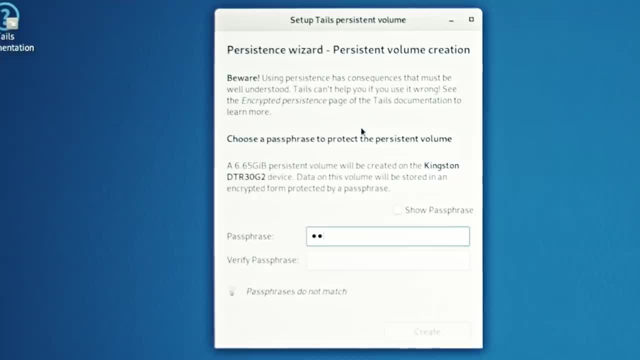 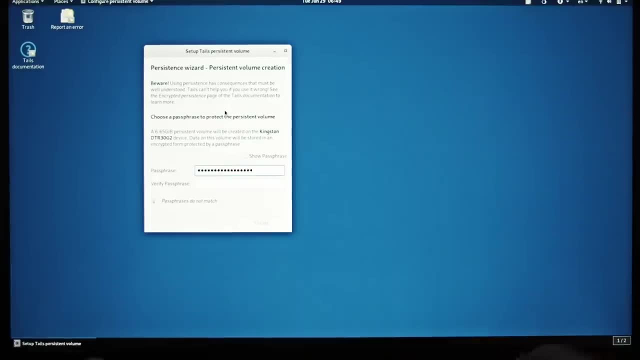 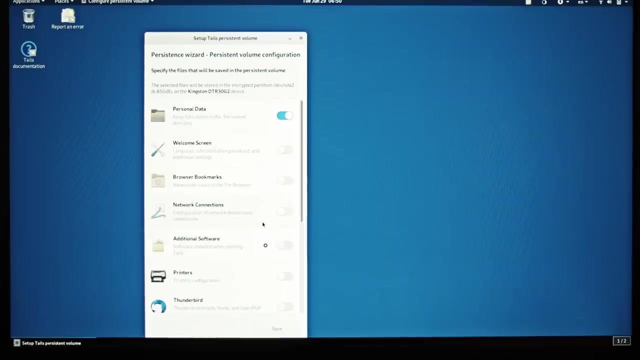 and might force you to reveal your password by a brute force attack to your knee. to create a persistent storage, choose applications tails. configure persistent volume. make a strong passphrase, verify it and click create tails. only recommend to activate personal data persistence feature for beginners. additional features can be activated.